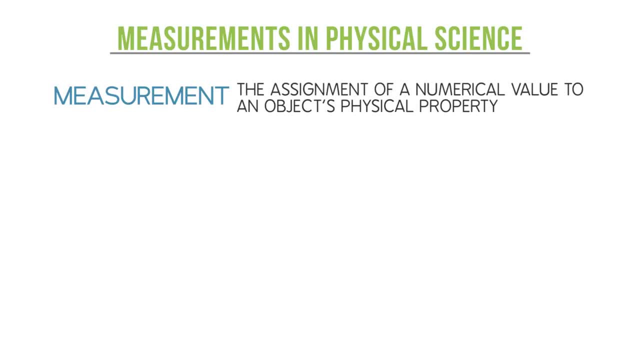 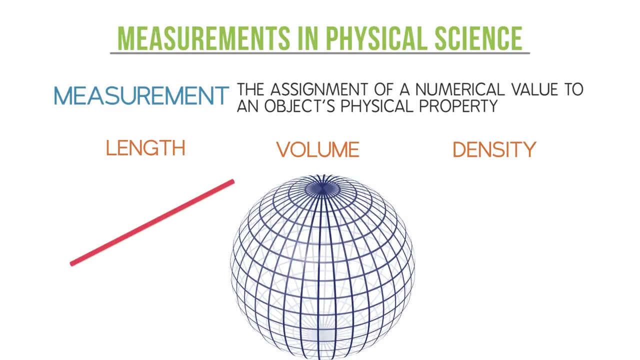 in science, a measurement is considered the assignment of a numerical value to an object's physical property. Measuring physical properties such as length, volume and density is very common. For example, you might want to know the length of a line, the volume of a sphere. 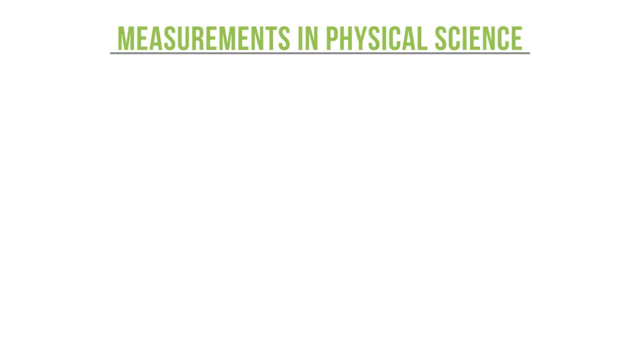 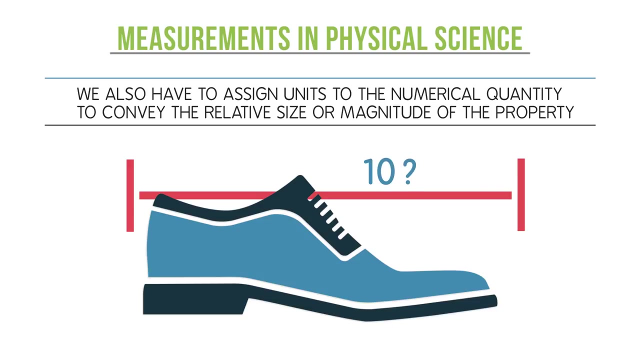 or the density of a liquid. Whenever we take measurements, we also have to assign units to the numerical quantity in order to convey the relative size or magnitude of the property in question. For instance, if I said the length of my shoe was 10, you wouldn't actually know how. 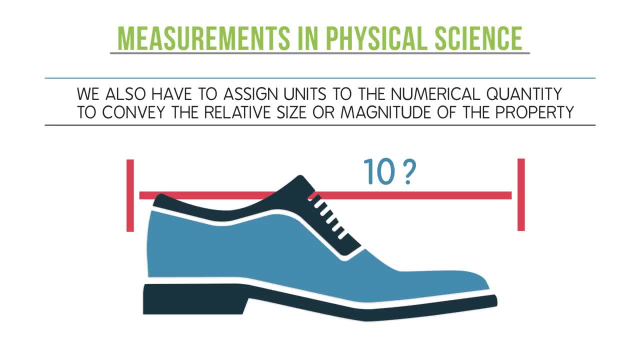 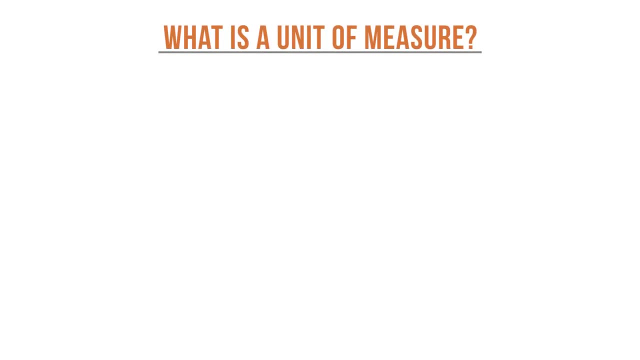 long my shoe was because there would be no context for what the 10 represents. In fact, this measure would only make sense if the number 10 had a unit of measure to go along with it. So what is a unit of measure, In order to have accurate and reproducible ways to define? 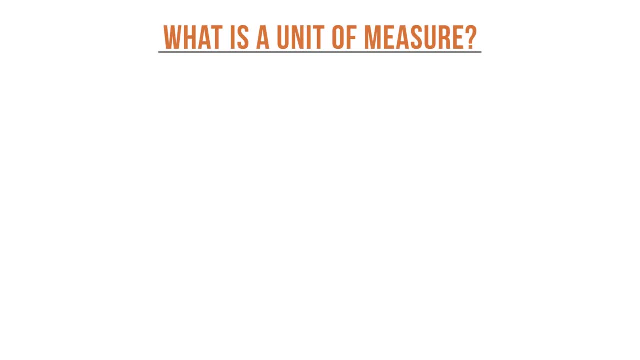 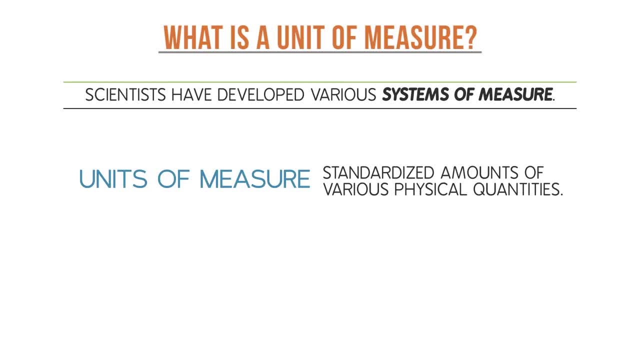 measure. These systems are made up of units of measure, which are basically standardized amounts of various physical quantities. The SI system is the international system of measure used by scientists. It is a very comprehensive system with many units of measure. However, we will only need to cover a few of these units in order to prepare for the T's. 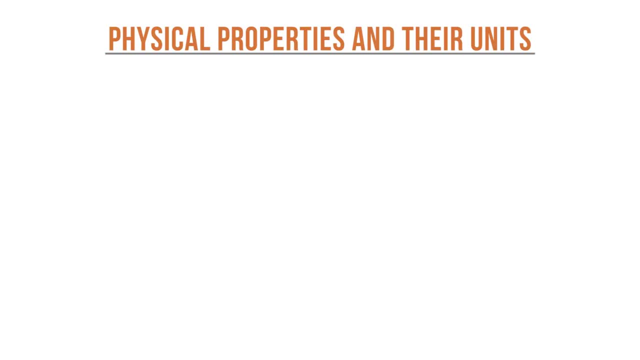 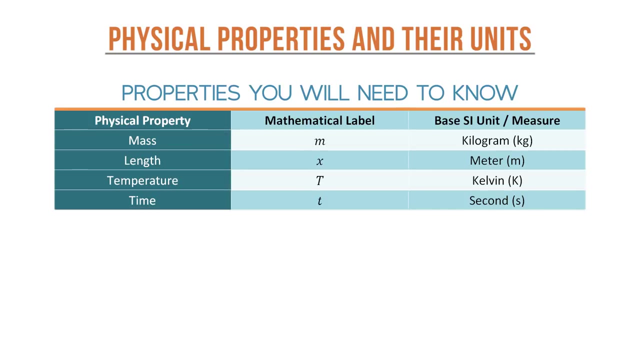 The fundamental physical properties you will need to know for the T's are as follows: Mass, length, temperature and time. You can see that for each property there is a mathematical label which is used in formulas and the actual name of the corresponding SI unit or measure. Please feel free to pause. 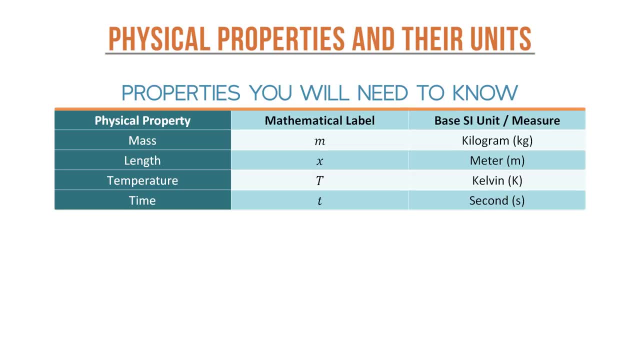 the video and familiarize yourself with the information on this chart. Notice that the chart refers to these units as base units because they help to define more complex units, which are called derived units. For example, area is a physical property, property that uses a unit called meter squared, Since meter squared requires the 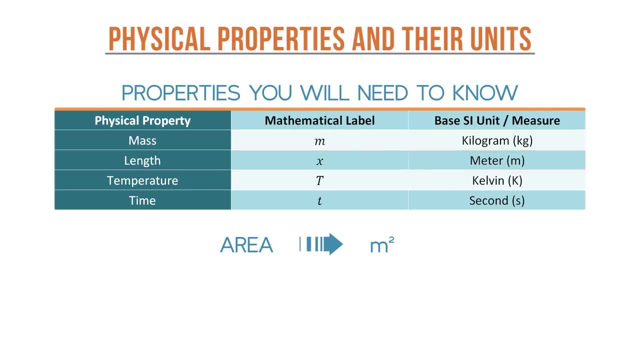 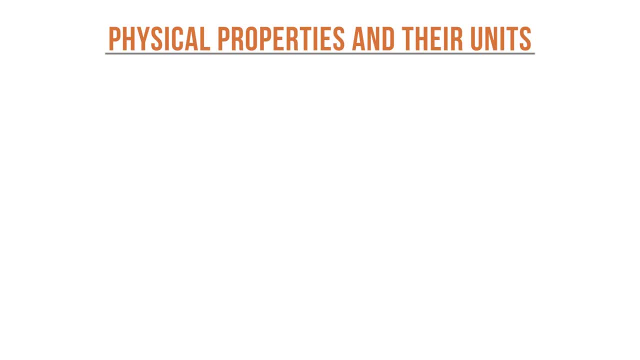 meter. in order to be defined, it is considered a derived measure or unit. Let's walk through an example that will illustrate how the meter is actually used to define area in meter squared. If we take a line that is two meters in length and then create a square from four of these same lines, we can find out: